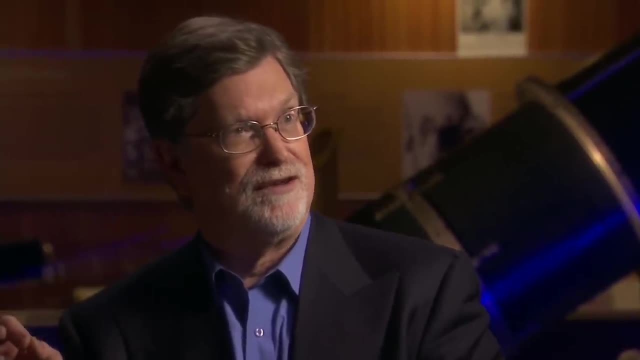 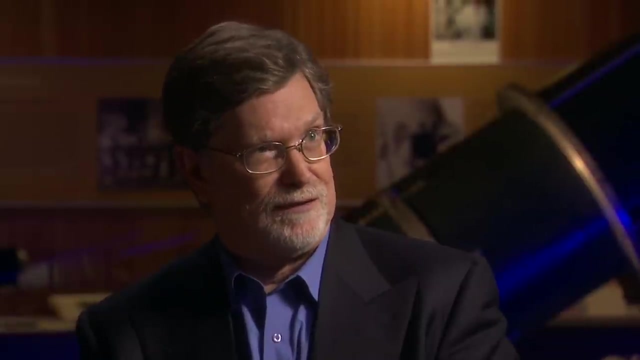 on the size of the galaxy. we think that we wasted 90% of our potential, And you can see that. Well, how fast does the sun go around the galaxy? Well, it goes around at about a thousandth the speed of light, a little less than a thousandth the speed of light. 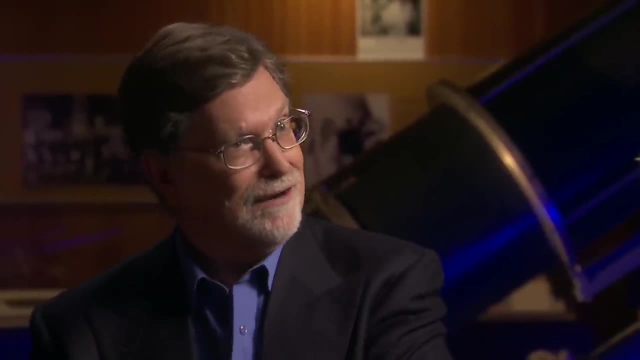 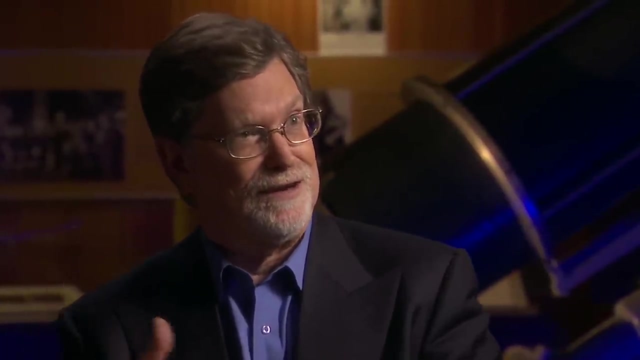 So if you remember your Newtonian physics, a half mv squared right. compare that to mc squared Right, right, right, Right. It's roughly a part in a million, and yet the variations are about a part in a hundred. 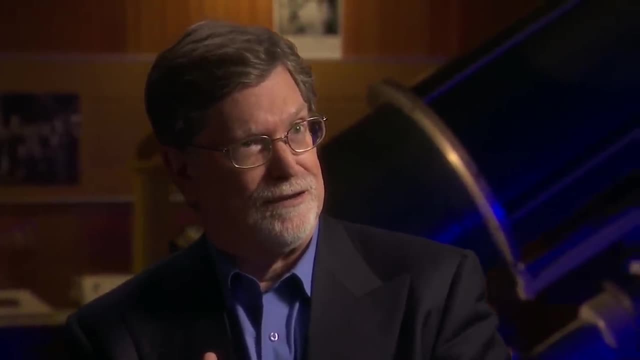 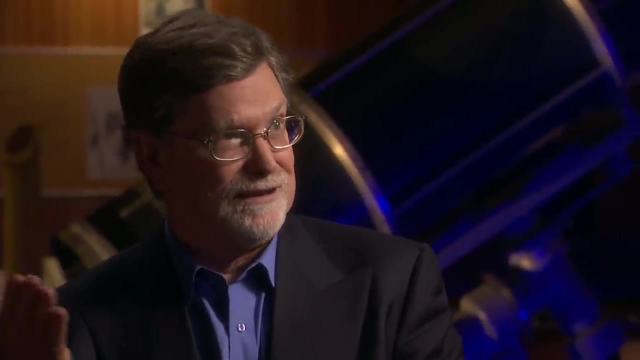 thousand right And so that we're in there to begin with the potential variations. So we wasted 90% of our potential to make the galaxy right. But when you get to clusters of galaxies they're up with almost their full potential. That is the part in a hundred. 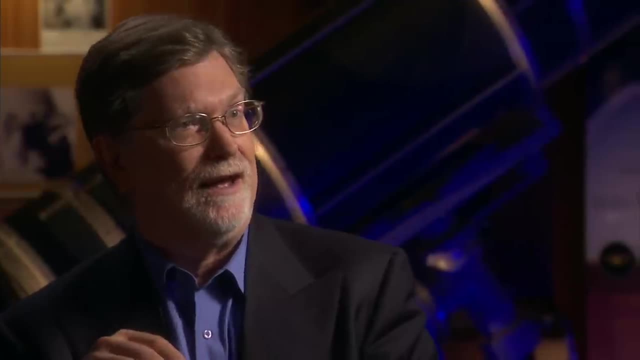 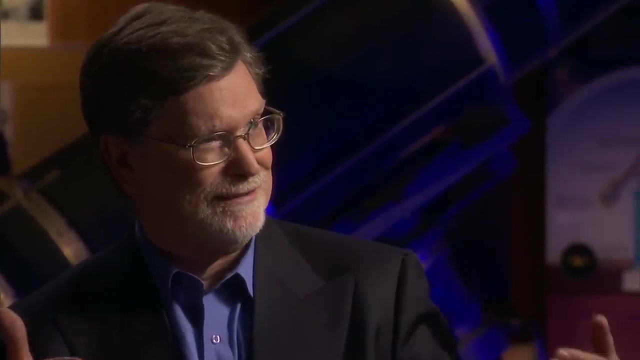 thousand. they're much, you know, bigger and more bound. And the other thing that's magic is that size of clusters of galaxies is the size where the sound horizon is, So that's where the potential is. There's a particular scale picked out, And so we expect. 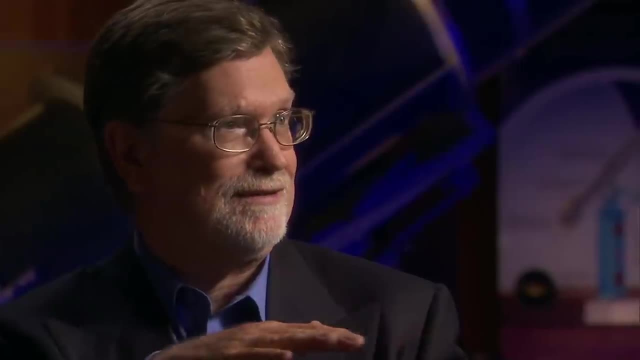 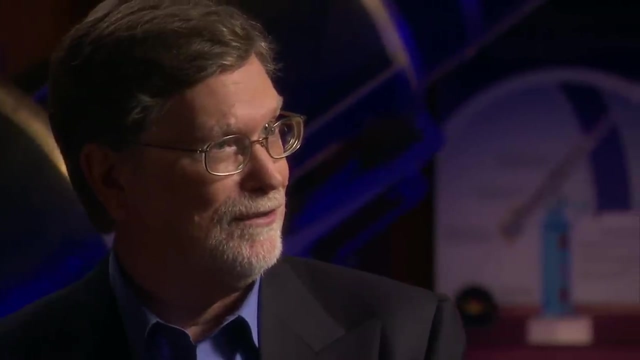 to see that there's roughly equal variations across the sky of all structural scales, till you get to the sound horizon, And then that's the part where you're dissipating away your potential. So then you get to the size of the galaxy. you only have 10% left, And when 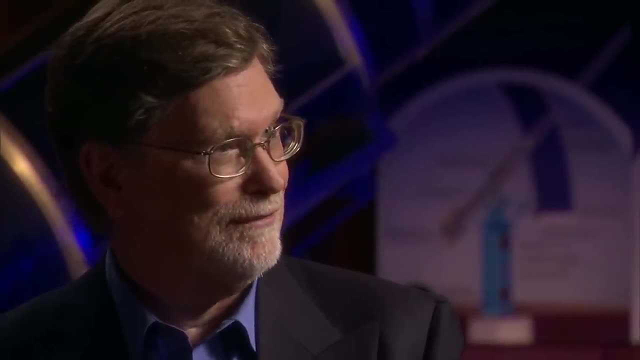 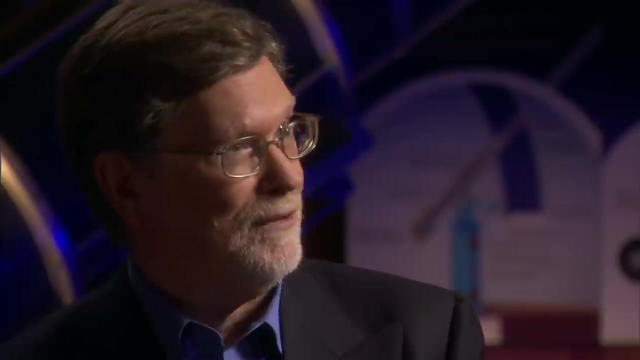 you get to the size of clusters- you know star clusters. you have only a smaller percentage left And you get down to the size of stars. that's all dissipated away. It's just random variations that we see stars in And we. so we can make up this map, We can do computer. 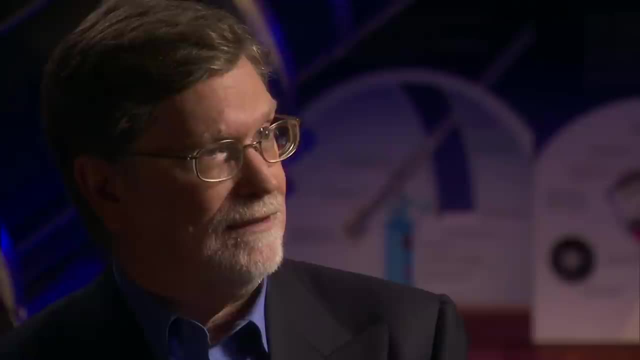 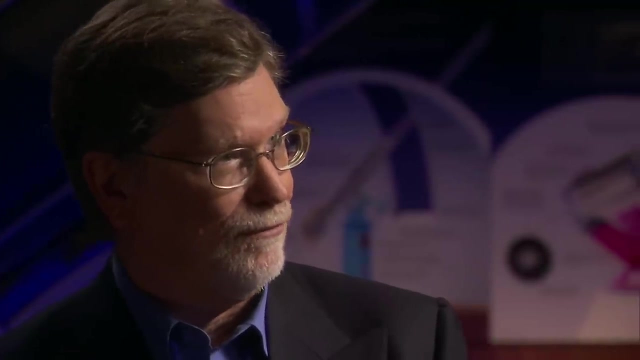 simulations And we see this evolution And the thing that has happened is the things that are really big. the matter hasn't had time to move around, So they're pretty much primordial And they haven't formed their large-scale structure. And because the universe is accelerating apart now. they won't ever get the chance to do that. But when you get down to the scale size of the Great Wall and then you know clusters of clusters of galaxies, they're the biggest things that will form, because now we shut off the formation of structure. 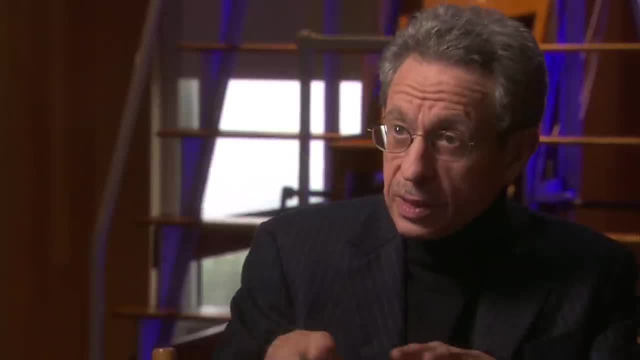 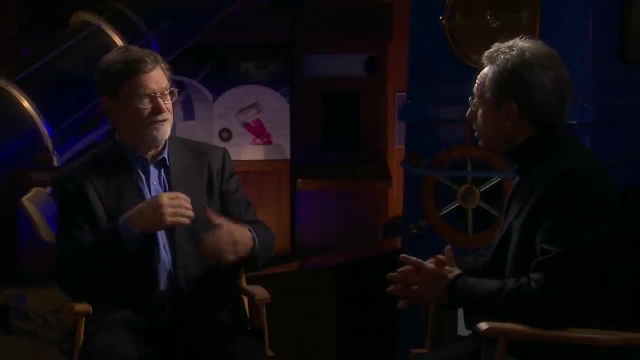 by the accelerating expansion of the universe. But what's particularly remarkable is that you can forecast all of this from the early universe, from the picture of the early universe. That's right. You can start with this very simple case, basically homogeneous soup, It's. 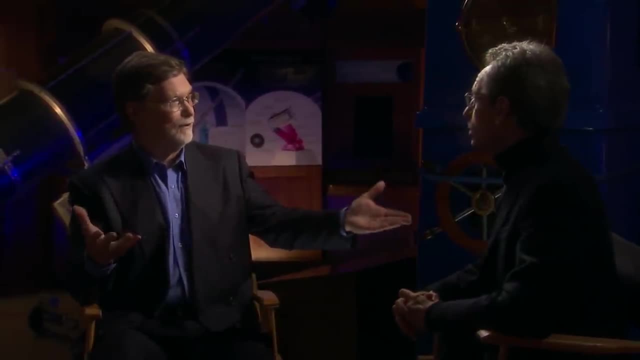 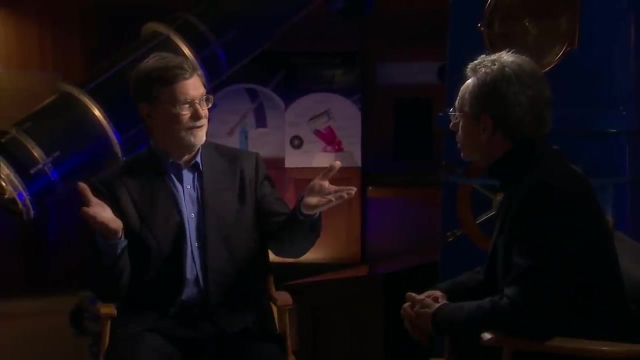 like a glass of water with just a few specks in it, And those are going to grow kind of like mold, except it's by gravitation absorption. You can do those calculations. You just need Newtonian gravity or Einstein gravity. It's simple, You just do the calculation, It's. 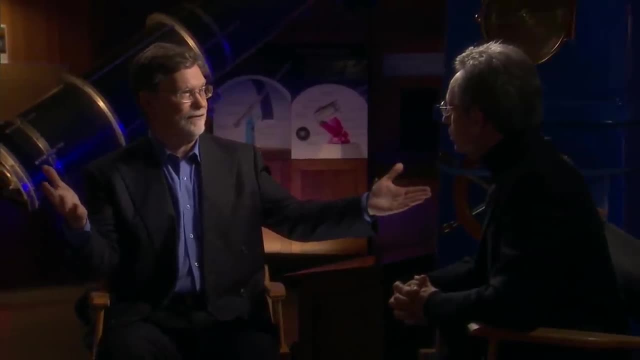 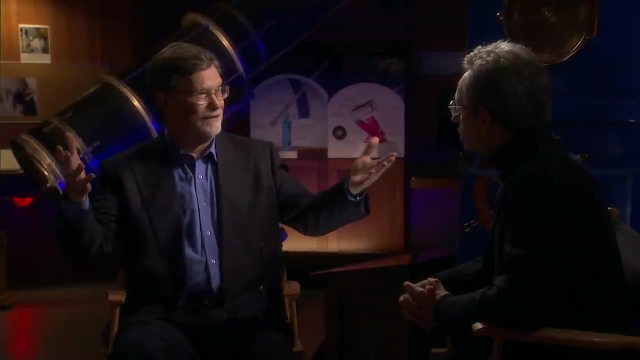 just a big calculation to do, because the universe is big. Even a section of the universe is very big. So you have these huge scales But you just start and you just let 14 billion years go by and gravity pulling it in, And eventually you'll find this, what we call the cosmic web. 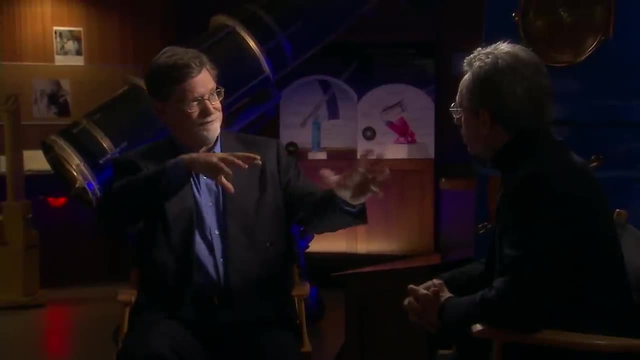 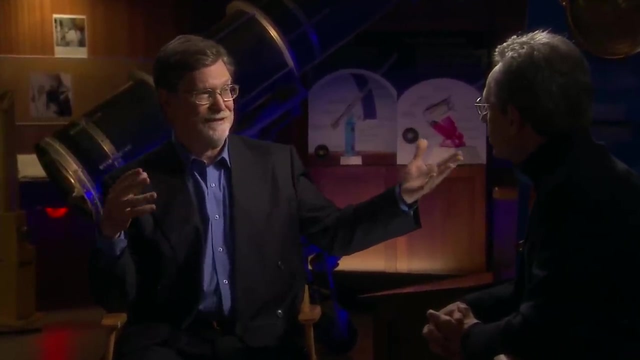 this structure where there are these large like dirty cobwebs of galaxies. You know they're beautiful, They're nice shining lights in the sky that are just. you know, take your breath away when you look at it. So I hope you put up the Hubble Deep Field. 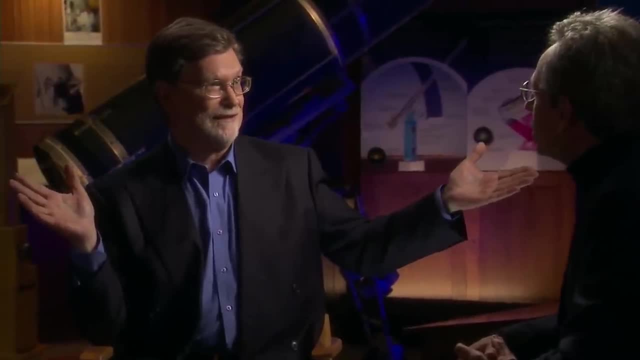 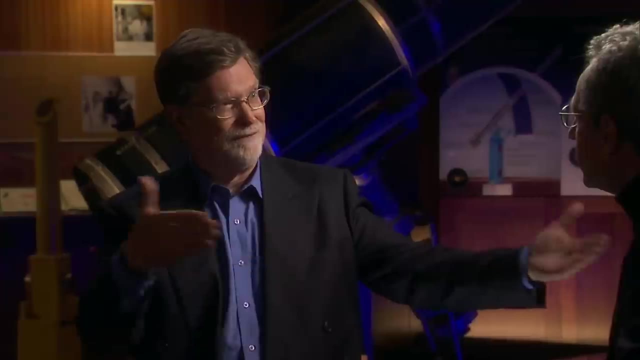 Yes, And it's just. you know, look at that picture and I see millions of galaxies in that picture and I go. you know, wow, Yeah, Either. one of those was a quantum fluctuation and it just got expanded by the expansion. 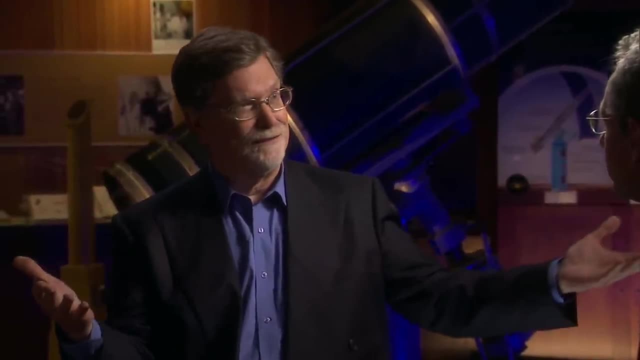 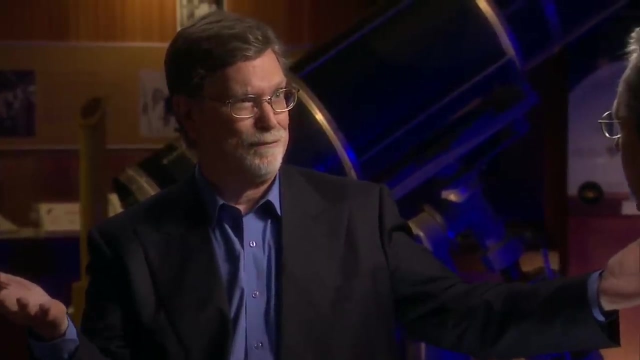 of the universe to be this scale, And then all you had to do was cook it for sort of let it cool on the stove, so to say, for the 14 billion years, And then you've got these beautiful jewels. It started. we know where it is now. these beautiful clusters of galaxies, We know that. 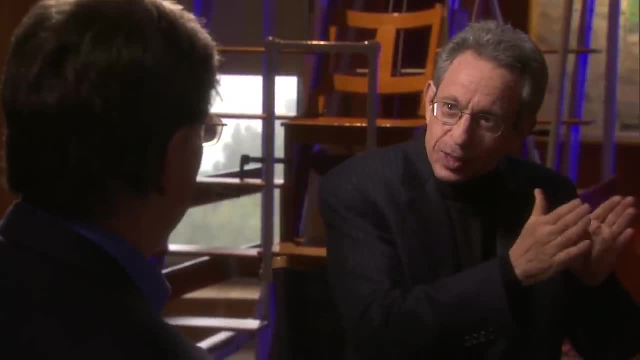 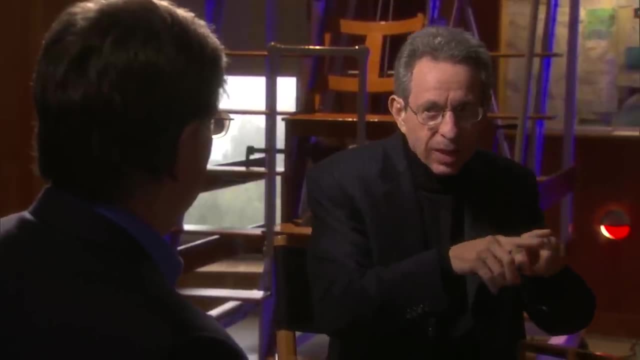 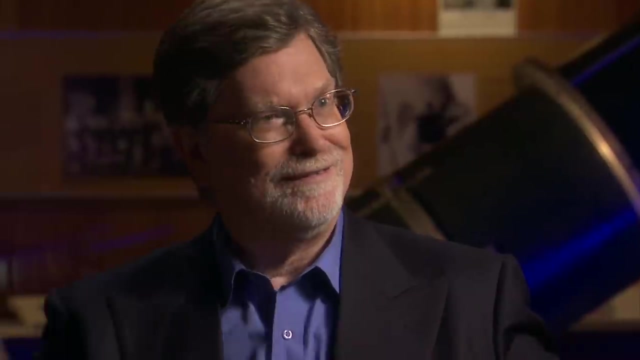 it started in this quantum fluctuation. But you then took this picture right soon after that quantum fluctuation, birth, Right, And it's that picture. that is not a theory, I mean, that's a real photograph. So it's a photograph and it's a number. It says: just put in, you know, scale, invariant. 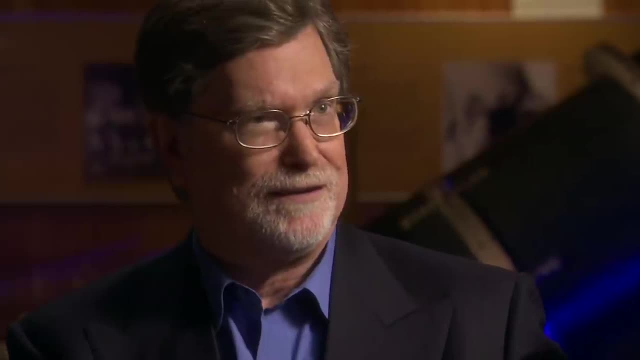 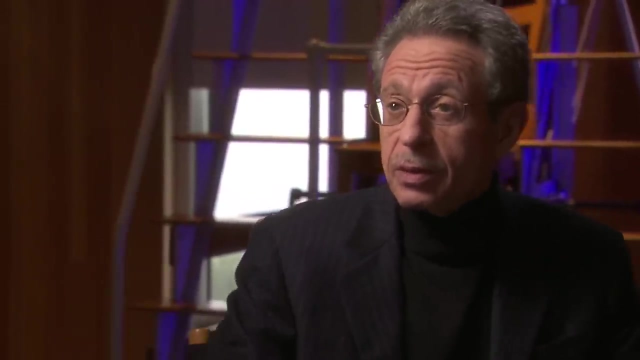 perturbations at this level, right, independent of scale. Just put them in at the 100,000 level, energy density variations and whammo, And then run your simulation. Yeah, Just run your simulation and you get… Based on gravity. 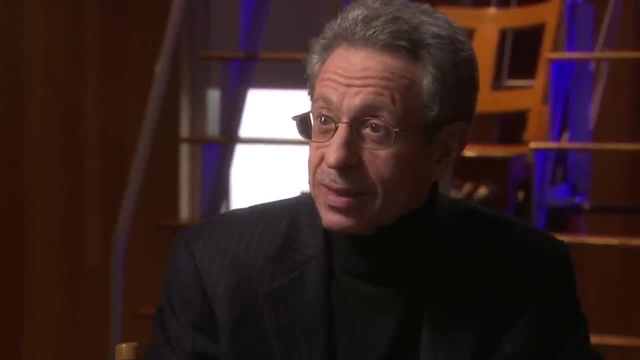 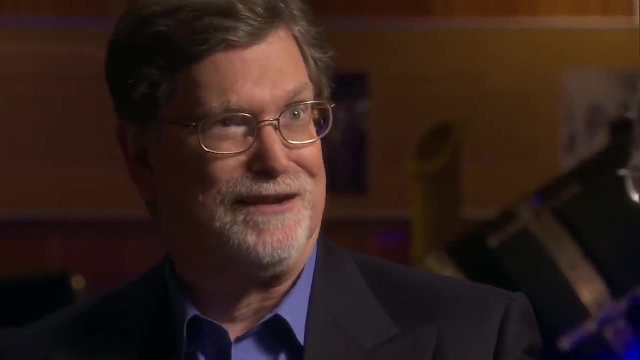 You get something that looks like the universe- Yeah, And just add time. It's like a little cookbook on how to make a universe- Add time, Yeah, And it only gets complicated when you actually start turning the stars and the gas on it. 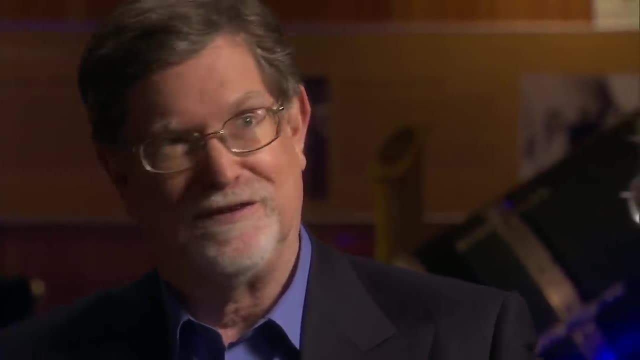 and so forth. Then you've got to be a little more careful about what's going on with the rest of it. Most of it's just simple linear calculations, Just a lot of number. you know there's a lot of particles, so you have a lot of stuff that you can work out. 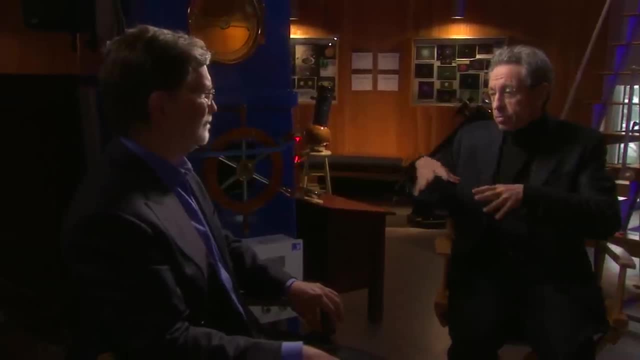 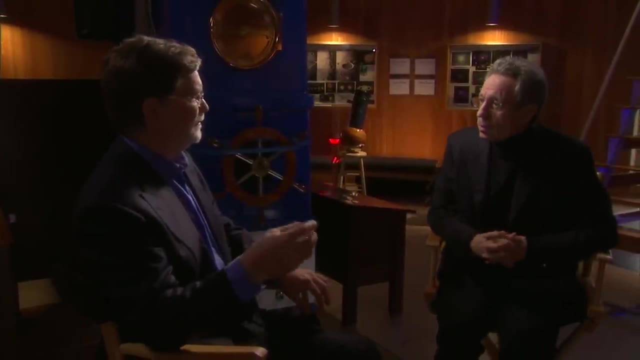 Right, right, right, And the large scale structure have the greater form, and then there's more variance in the individual stars As you get down, smaller. yes, then you've gotten to the nonlinear part where things have clumped up and formed these beautiful spirals, or the ellipticals. 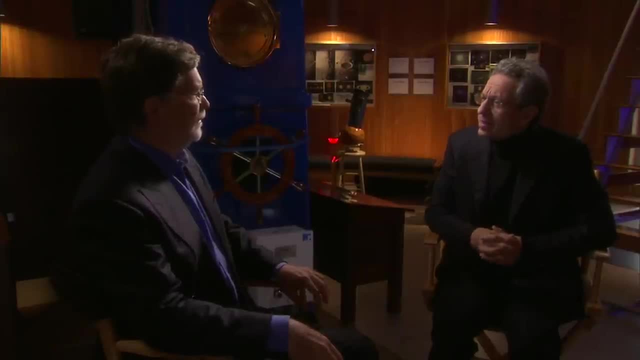 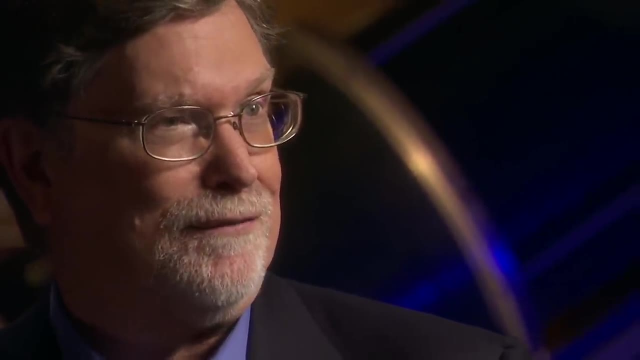 Could I ask you a question? Could it have been any other way? Well, of course, I mean you can imagine. Suppose you thought that you just had to make a place for people to be. Well, a galaxy is plenty big, right, I mean. why would you make? 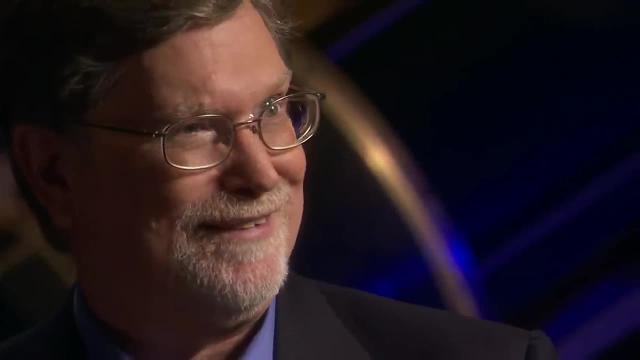 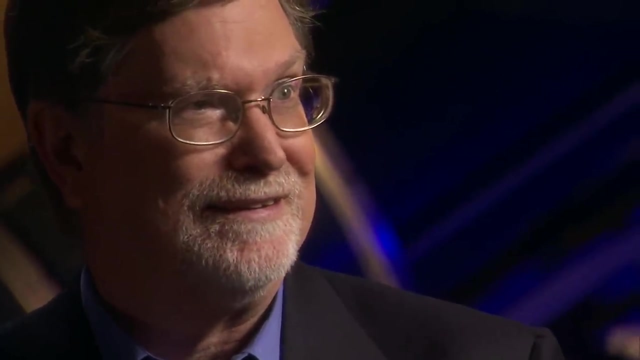 hundreds of billions of galaxies. right? Why would you? you know, of course, you could have made it different, right? It could be an island universe, It could be just the solar system by itself. right? I mean, you could have made it much different. You could have had a universe. 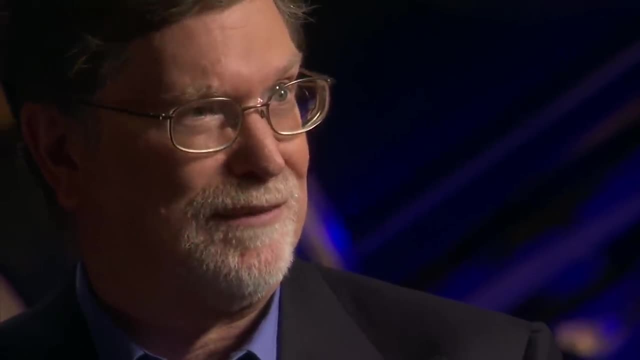 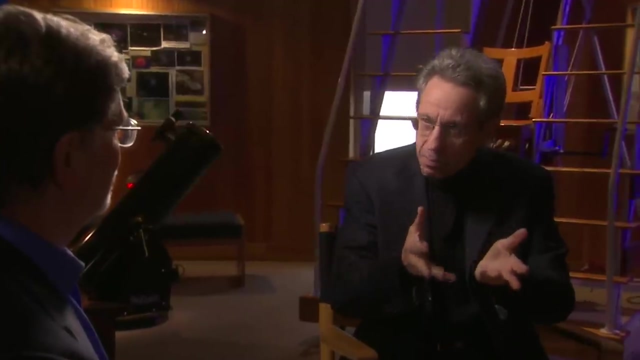 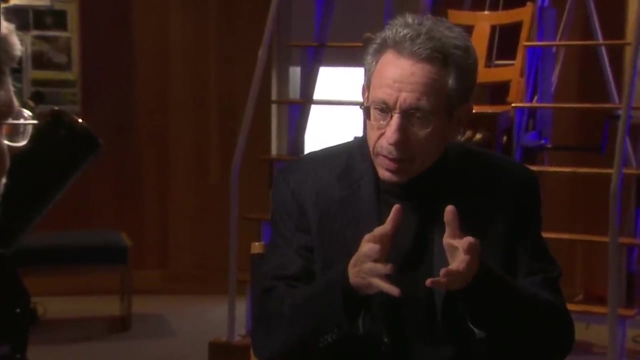 that existed for a second and collapsed right. There's a lot of other possibilities, But to generate the kind of universe that we have today, how else could that? might that have been done from the early universe? To get something like today? I mean how fine-tuned. 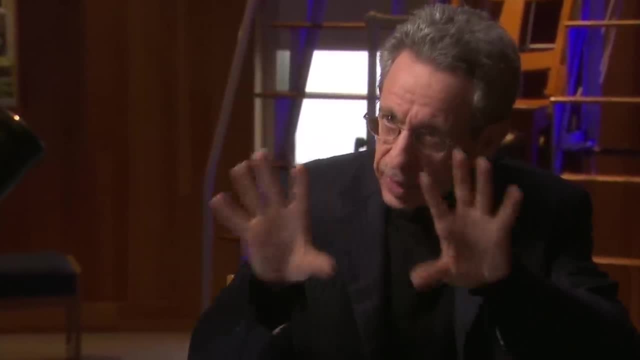 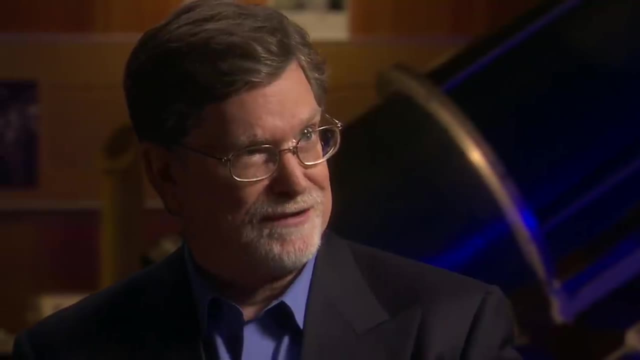 is the term. Must that cosmic microwave picture be at that moment? This is interesting to speculate. what the real? you know what went on. So we have now a macroscopic description of what goes on. That is we know, just like we know the ideal. 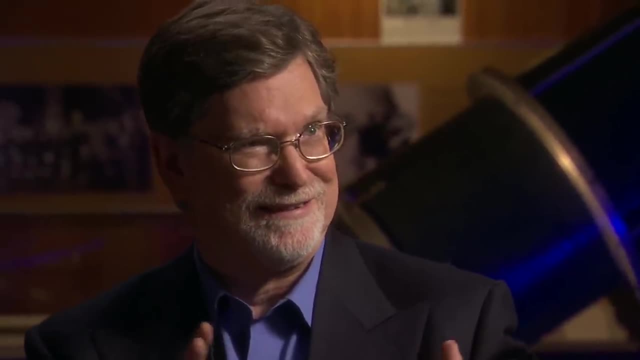 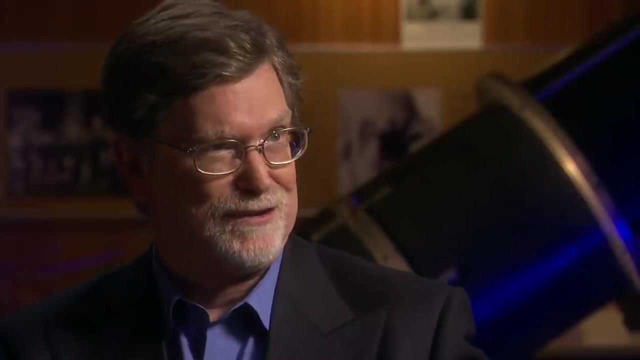 gas law right That if you pressure a gas that you know you make the volume, the volume will go down and so forth. It keeps the temperature constant. Or you keep the volume constant and you put pressure the temperature you know so forth. So you know that as a macroscopic. 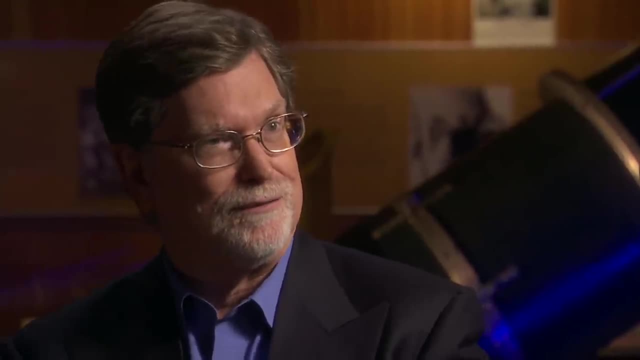 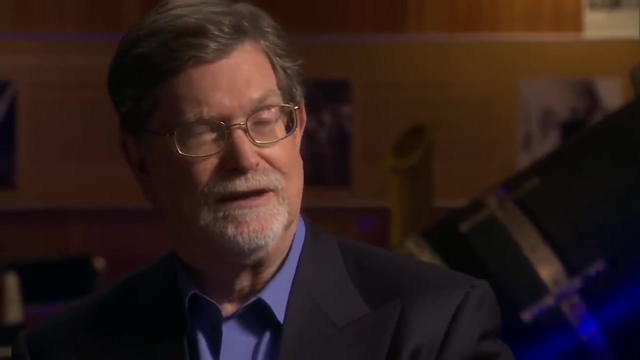 law, You start understanding it microscopically. when you start thinking molecules are moving around and they're colliding with each other at random, You can sort of understand how that macroscopic law you can derive it very directly. So we're in a situation where we 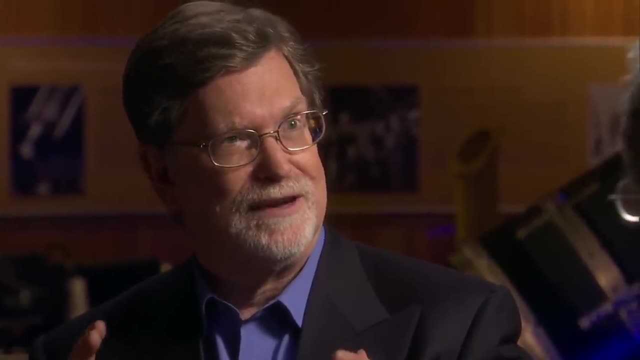 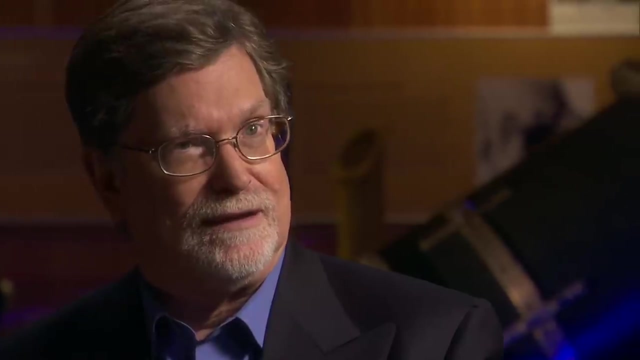 understand the macroscopic universe in a very well. Now we're trying to understand what's the detailed, microscopic description of what happened. So the answer to your question is no. it could not have happened in a different way because we have all these needles You've. 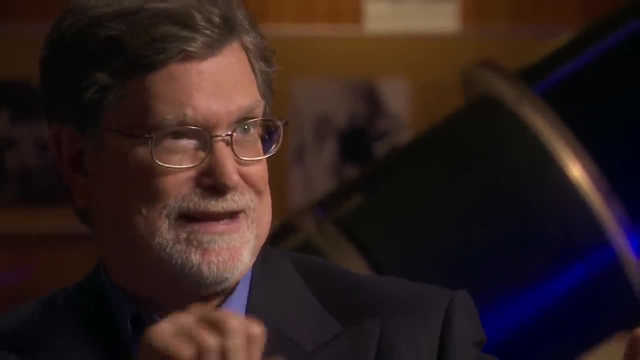 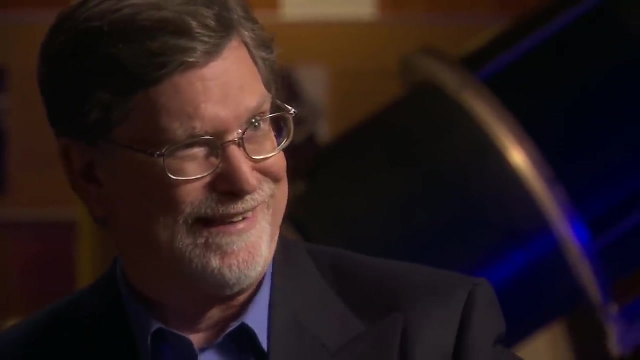 got a thread right. You have these observations that tie you down very tightly about how the universe itself actually evolved, But you can imagine different scenarios that lead you through that needle, right. I mean, there's room for the thread to wiggle around a little. 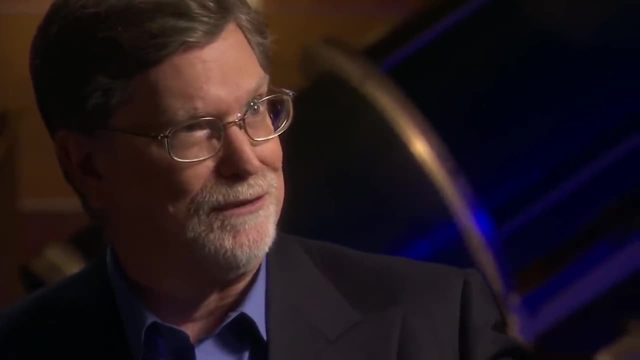 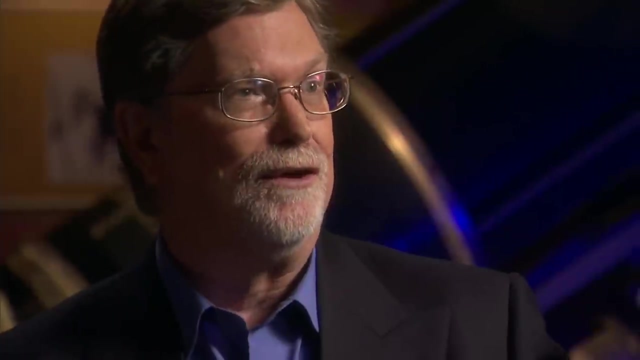 bit, But not too much, in the later universe. The early universe is where the loose ends are flopping. That's when you get to string theory or to extra dimensions and brain inflation, Those kind of things. they also got to sneak down and fit through these observations.